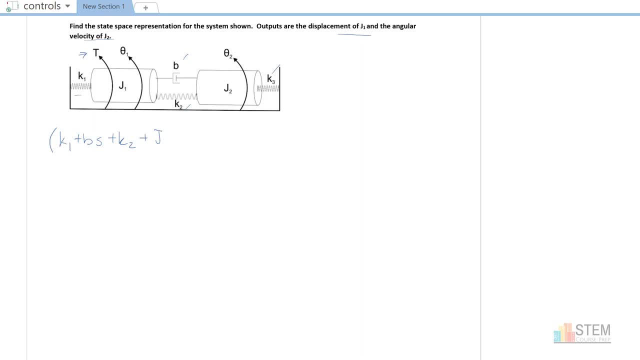 going to need to include that. So we're going to have plus J1 S squared. Now all of those need to be multiplied by theta 1 of S. Next we want to look at the interaction impedances. So these will be negative. So put that negative here, And then what we want to do is find: 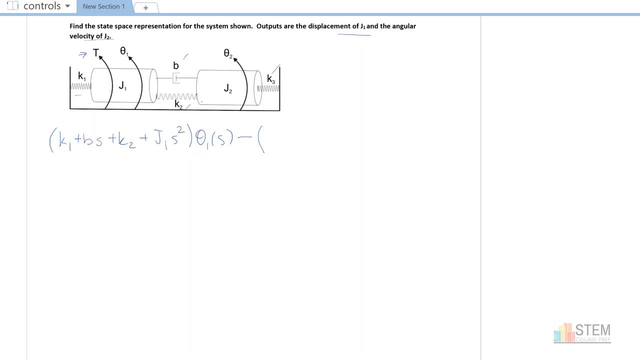 everything that connects the two cylinders. So I've got B and K2.. That's all we need in this term here. So we're going to have a damper, We're going to have B times S, And then we're going to. 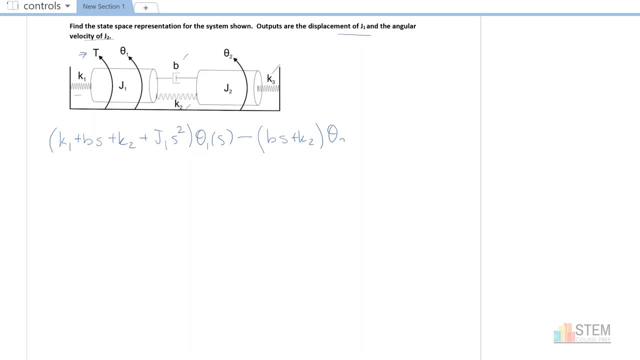 have plus K2.. Multiply that by theta 2 of S, And then, finally, the right side will equal the applied torque on J1, which would just be T of S. All right, so let's call this equation 1.. Now let's go over to the second cylinder. Now I'm going to keep these in the same order. 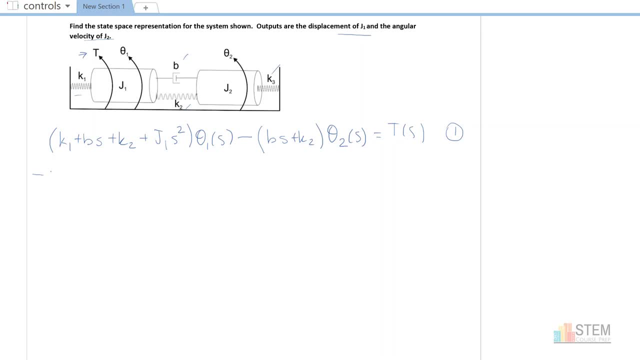 where theta 1 is the first term. So for this equation, since this is the equation for J2, this will be our interaction term, So this needs to be negative here. So again, pull off everything that's going to basically connect the two cylinders together. 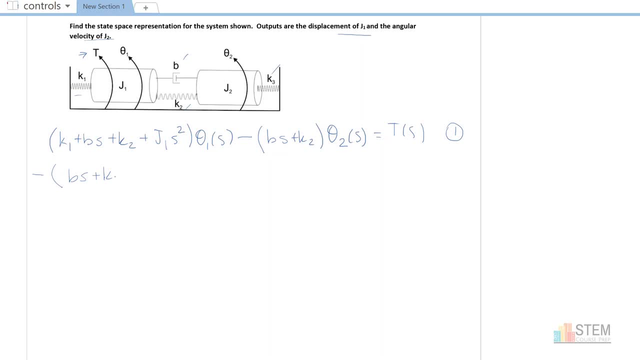 So we're going to have BS plus K2.. Multiply that by theta 1 of S, Then we go to the theta 2 term. So now you want to look at every element that's going to create a torque when we have motion. 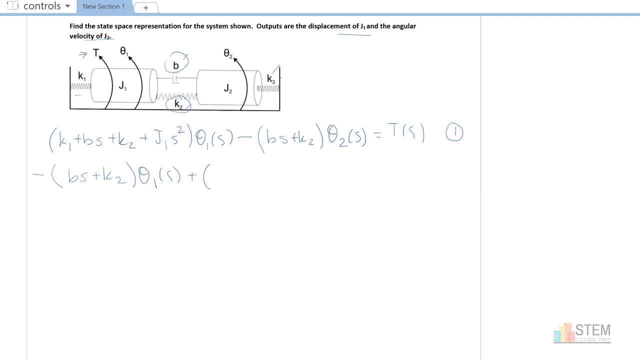 So that would be this damper this spring, this spring, And then you have the inertia itself. So we're going to have B times S plus K2, plus K3 plus J2.. And then we want S squared on that J2 term. 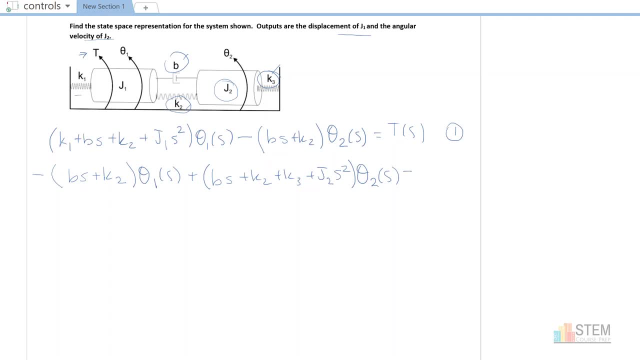 And then multiply that by theta 2.. And then multiply that by theta 2 of S. Now this right side will be 0, because I don't have an applied torque on J2.. So now we've got that OK. so let's call this equation 2.. 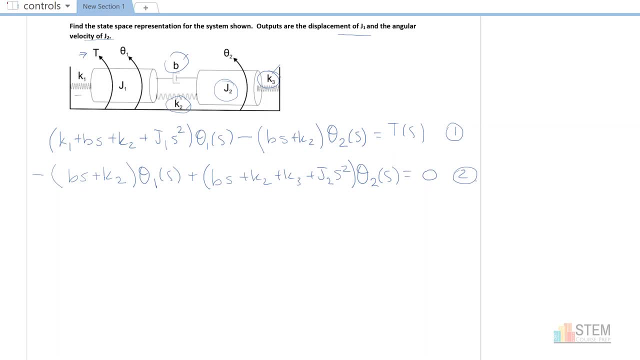 So we went through and we got those two equations. that didn't take much time at all. Now what I need to do is get this in terms of T. I need an actual differential equation. So all we're going to do is kind of go backwards here. We're going to take this equation 1.. 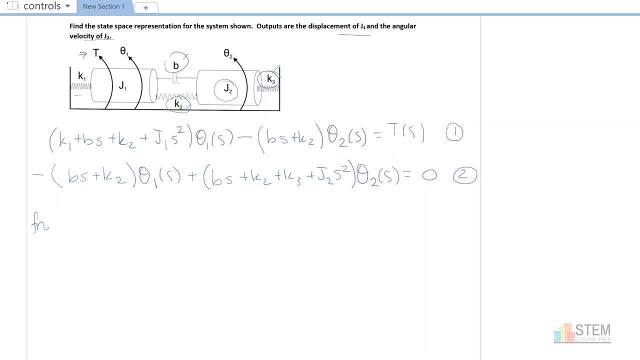 And basically do the inverse Laplace. All right, we're assuming 0 initial conditions here. So if we do that, we're going to have K1- theta 1 plus B- theta 1 dot, And I know this is theta 1 dot because we have this S here. 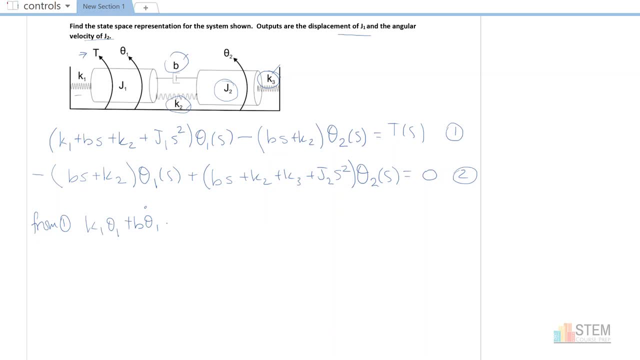 So it would be S, theta 1.. So when you do the inverse Laplace, you get that theta 1.. And then we'd have plus K2, theta 1.. And then 5, theta 1.. finally, plus J1, theta 1, double dot. Now we go to the next one. So minus B, theta 2 dot. 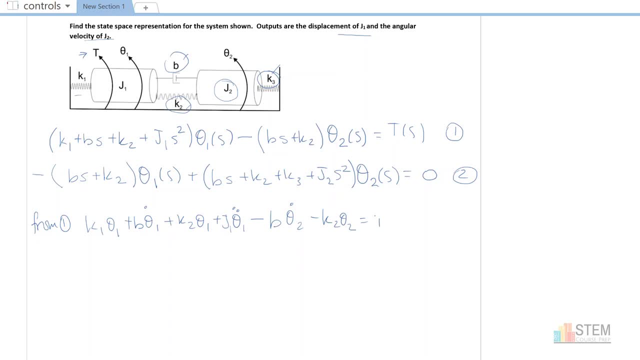 minus K2 theta 2, and then that's going to equal just your torque T, All right, so now we have that And then, if you want, at this point you can group up your terms. All right, because we have two theta 1 terms, so let's group those up. So we'll have K1 plus K2 theta. 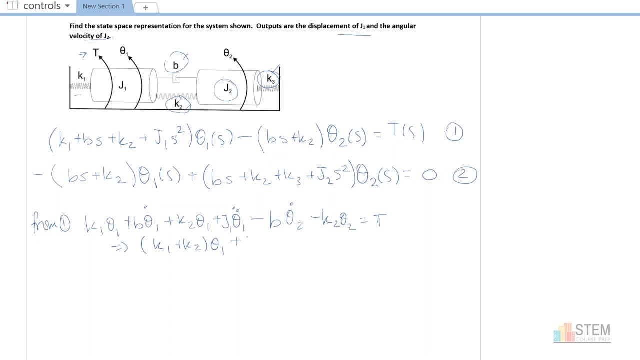 1, and then you got your theta 1 dot here. So B theta 1 dot, and what else do we got Plus K2 theta 1.. Oh, actually, we already had that one. Forgot about that, Let's mark. 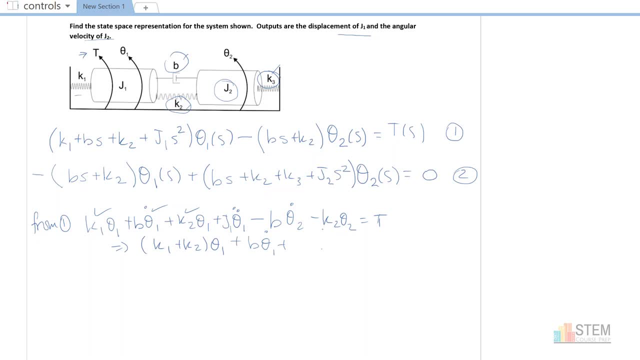 these off, So we have this, We have this and then the rest of them. you know, we can just basically put them in here, So just rewrite them, Okay. so now we've got that. Now what I want to do, because I'm doing- 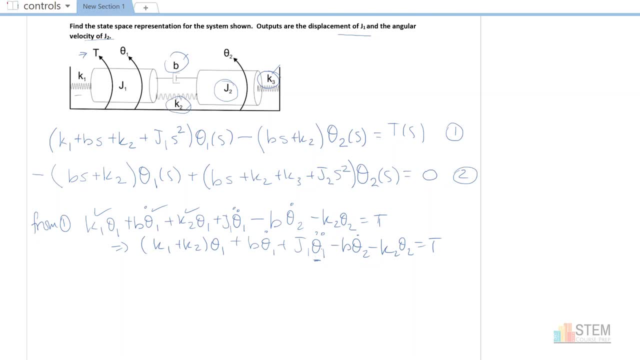 state space. here. I want to go ahead and solve this equation for theta 1 dot, because that's what we're going to need. Actually, it's theta 1 double dot, So I'm going to go ahead and do that. So if we do that, we're going to take everything else. move it over to the. 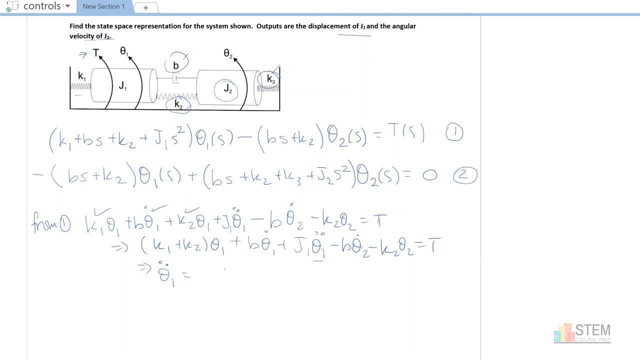 right, except for the theta 1 double dot, And if we do that, we're going to have the 1 over J1.. Let's put a bracket, We'll have T. I was going to put T of T, Let's just leave. 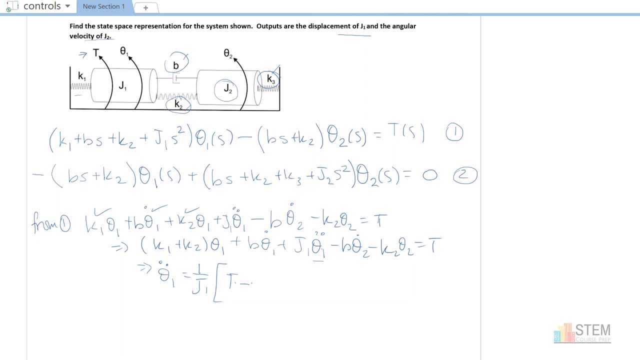 it as T, And then we're going to have minus K1 plus K2 times theta 1, minus B, theta 1.. theta 1: dot plus B, theta 2, dot plus K2, theta 2.. And this will be the equation we're going. 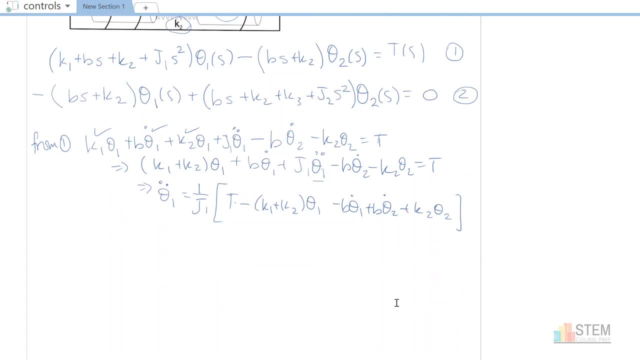 to use for state space. All right, now let's go and do the same thing for equation 2. And let's call this equation 3.. Okay, so same thing. We're just going to go through here. Anytime you have a variable multiplied by S, you know that's the first derivative of. 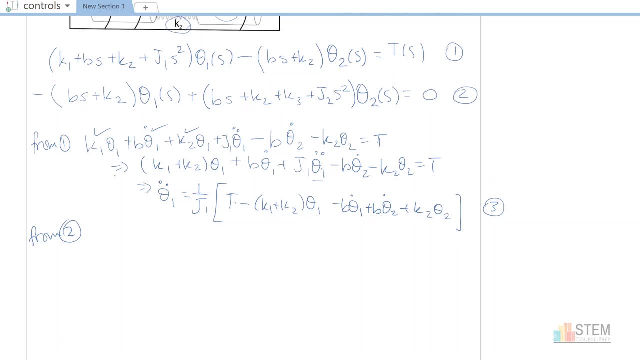 that theta term. If it's multiplied by S squared, it is the second derivative. So we're going to have negative B theta 1 dot minus K2 theta 1 plus B theta 2, dot plus K2. theta 2 plus K3 theta 2.. And then J2 theta 2, double dot. That equals 0.. 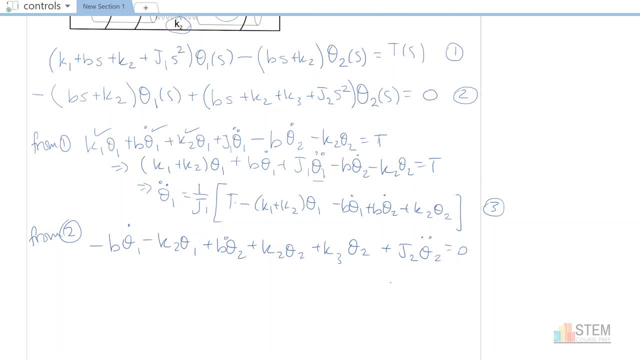 And now with that we can group up our terms. Notice, these two here can go together. And then we want to solve for theta 2 double dot. So I'm going to put those two steps together. So let's solve for theta 2 double dot and we'll put these two terms, the K2 and K3 terms. 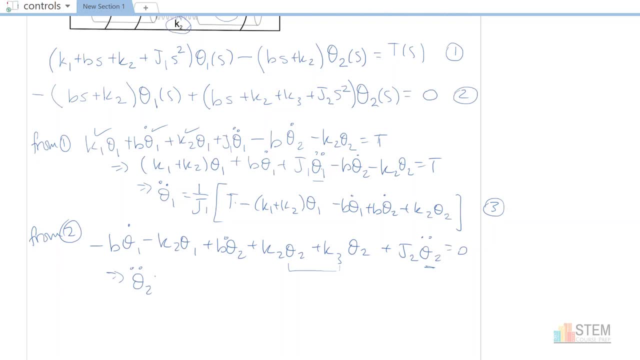 together. All right, so theta 2 double dot. we're going to divide through by J2.. And then we're going to move everything else over, so we need to switch the signs around. All right, so we're going to have B- theta 1 dot plus K. theta 1 minus B. theta 2 dot minus the. 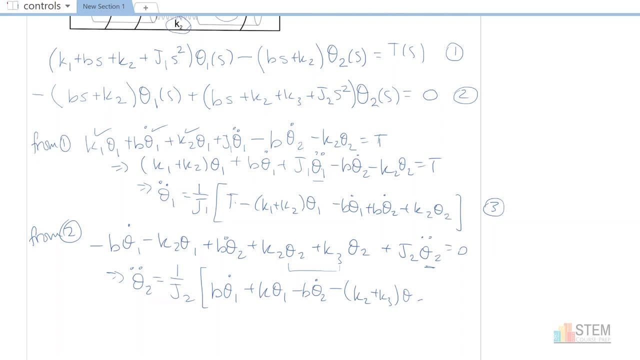 K2 plus K3, group those terms together, times theta 2.. And there you have that All right. so now we've got that ready to go, Let's call this equation four. So we're going to use three and four to get our state space. Now that we have that, the next thing. 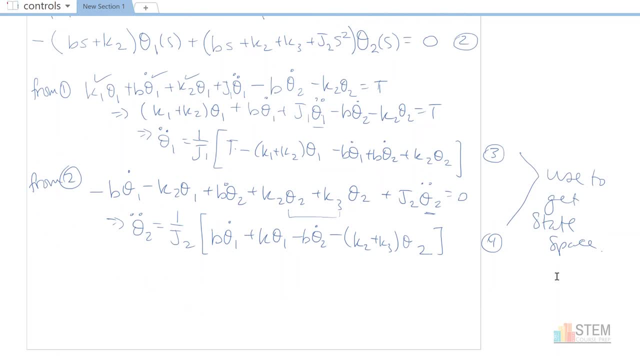 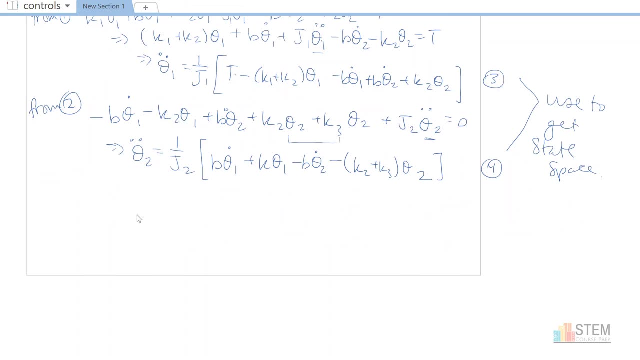 we need to do? we need to basically create our state vector. Now, for each thing that has an inertia or a mass, you need a variable for position and then for velocity. So in this case we have two j values, two inertias, so we're going to have four variables, right, and I'm going to call my 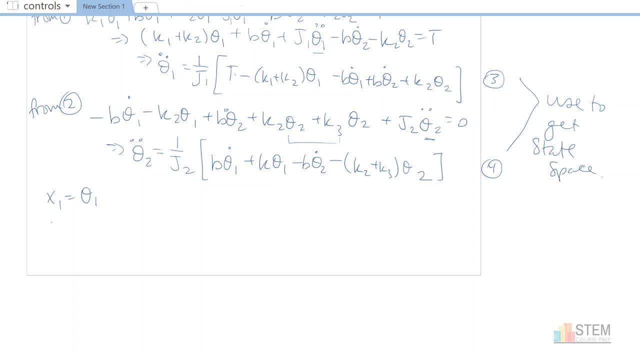 variables x. so x1 will represent theta 1, so that angular displacement of that first mass, and then we've got x2, that'll be theta 1 dot, so angular velocity there of j1, and then x3 will be. 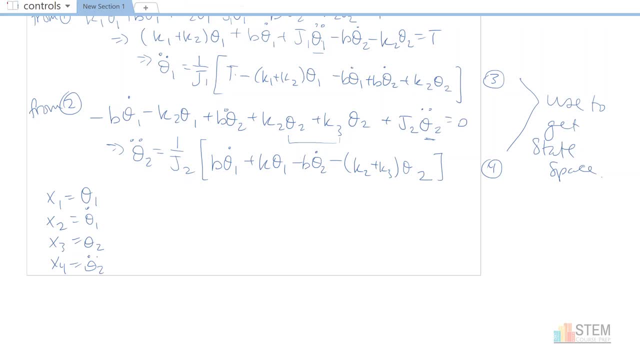 theta 2, x4 is going to be theta 2 dot, so these last two take care of the displacement and velocity for the cylinder j2.. Now what we want to do is we want to take the derivative of all of these and then we want to write everything in terms of x1 through x4, so we're going to have 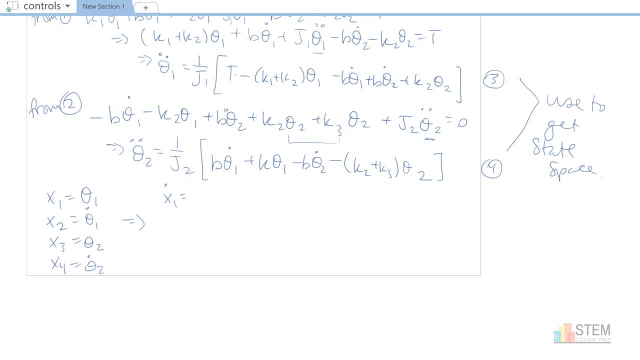 x1 dot. well, if I do x1 dot, then that means that's going to equal theta 1 dot and theta 1 dot. so that's going to equal theta 1 dot and theta 1 dot. and then we're going to write. 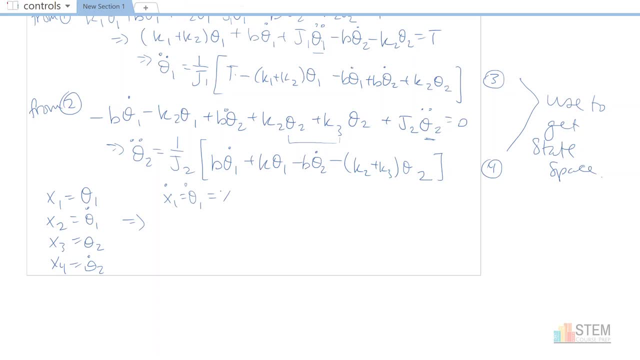 x1 dot. so we're going to have x1 dot and then we're going to have x1 dot, and then we're going to. one dot is equal to x2, all right, so we got that x2 dot. that gives me theta one double dot. 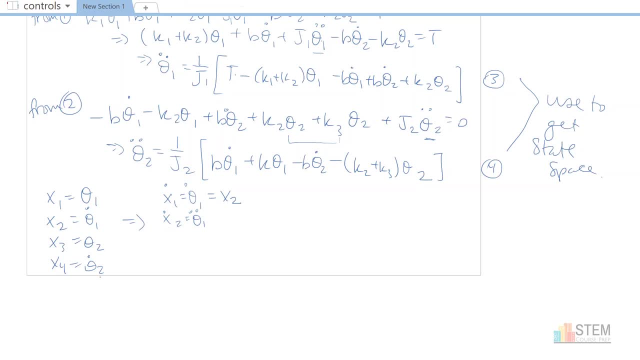 now I don't have a variable here for theta one double dot. so that means we're going to go up to our equation three right here and use that, and we're going to rewrite everything in terms of our little system variables. so instead of putting theta one and theta two, I'm going to use you know. 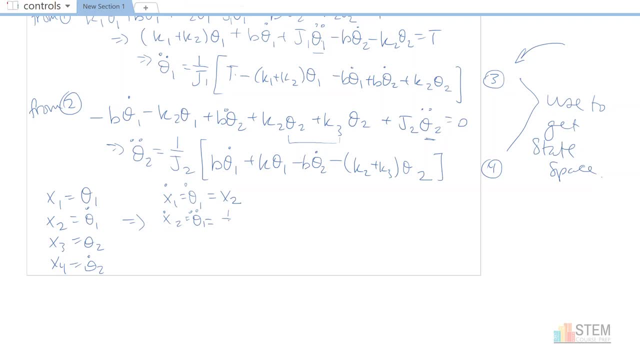 the x terms. so here we're going to have one over j one and we're going to have that times t minus the k1 plus k2. instead of theta one we're going to put x1, because theta one is equivalent to x1. so we got that. and then we need minus b theta one. 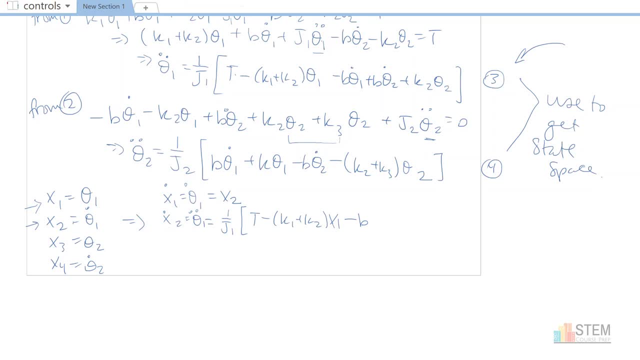 dot. well, theta 1 dot, as it says right here, is x2, so let's put minus b, x2, then we have plus b, x2, dot, x2, dot is x4, so plug in x4, and then, finally, last one, we have plus k2. 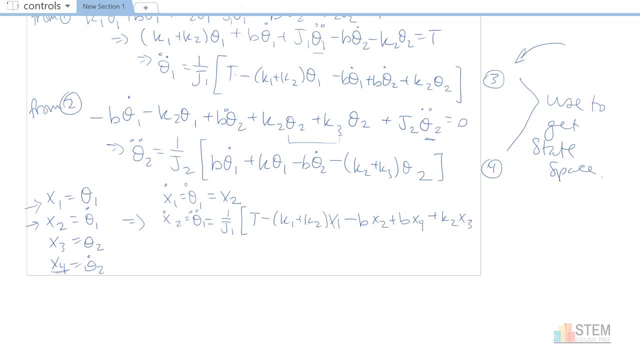 times theta 2, theta 2 is x3.. Next let's do x3 dot. well, x3 dot is going to be theta 2 dot, and theta 2 dot is x4, and then, finally, x4 dot is going to be x2, double dot. 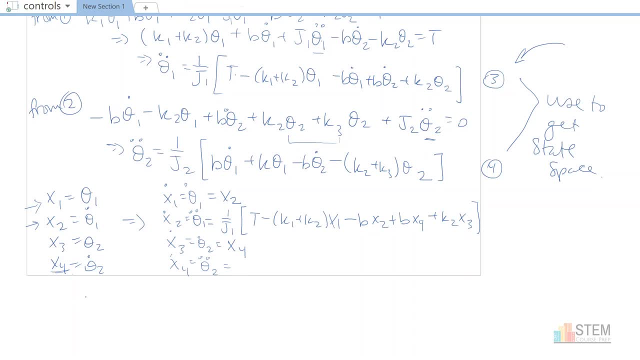 we don't have an x2 double dot variable over here, so we're going to use equation 4.. And if we do that, we're going to have 1 over j2 times b. now I've got theta 1 dot here. 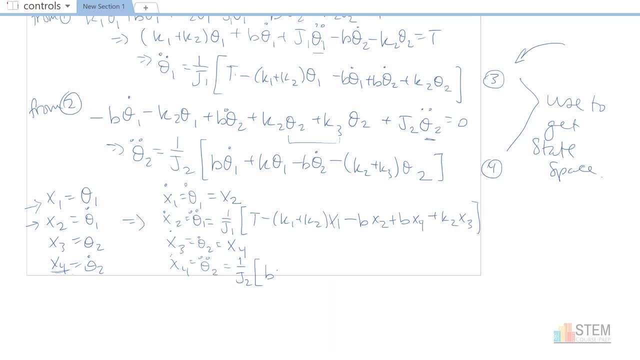 I don't want to leave that theta 1 dot. I want to change it over to x, so we're going to have x2, then plus k times theta 1, but theta 1 is equivalent to x1, minus b times theta 2 dot. 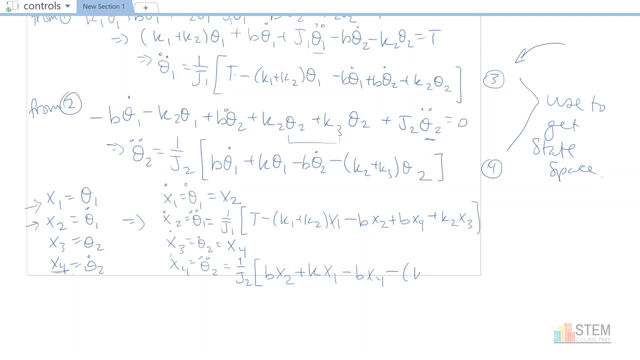 theta 2 dot and then minus b times theta 1, and then minus b times theta 2 dot. minus b times theta 1, minus b times theta 2 dot is x4. Then we have our negative k2 plus k3 term and then theta2 will be replaced with x3.. 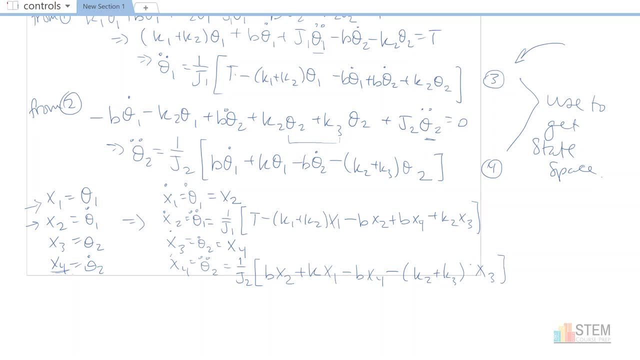 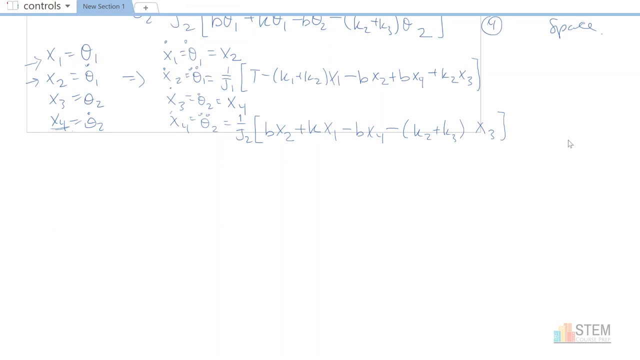 Once we're done with this, we're done with the hard part. Now we just have to basically pull off the coefficients and put them in those matrices. So, remember, the form we're going to have is going to be basically x dot equals ax plus b times u. So the left side will basically be: 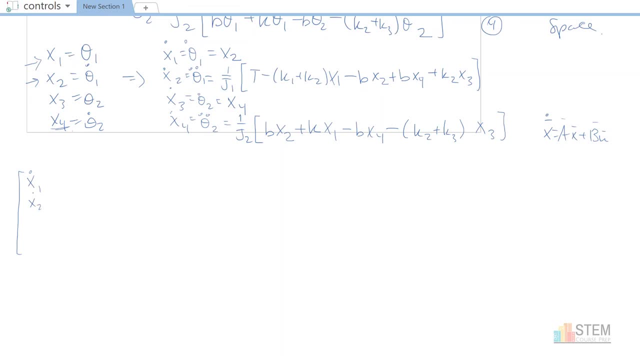 a column vector where we'll have x1 dot, x2 dot, x3 dot and x4 dot, And then we need matrix A. All we need to do to get matrix A is pull off our coefficients. All right and remember. 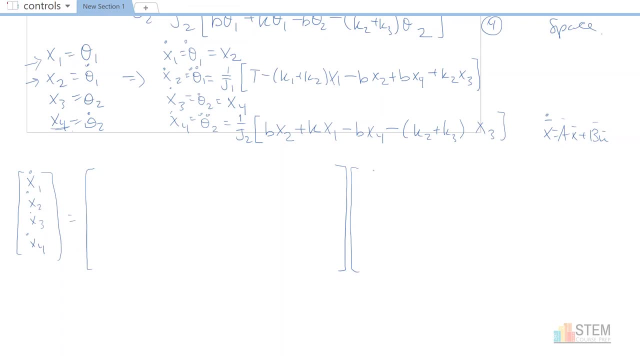 hopefully that leaves enough room there. Remember, we're multiplying A by our state vector, which would be x1,, x2,, x3, and x4.. Now let's start with the top row And I'll fill in the b times u at the end. I always do that last. 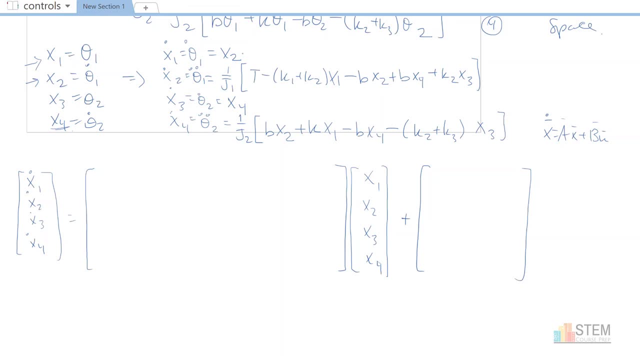 Okay, so our top row here we have x2.. So x1 dot is equal to x2.. So that means when I multiply through over here, I'm going to have 0, 1,, 0, 0.. Because that way when I multiply these vectors, 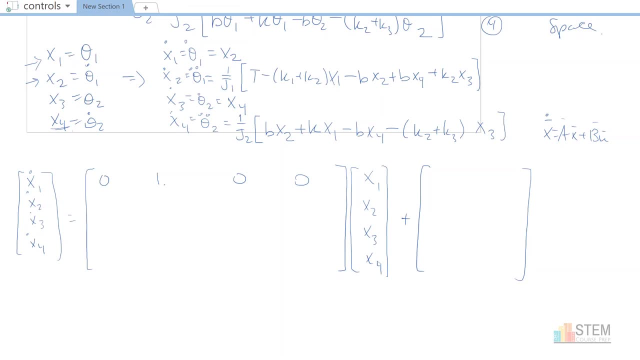 or matrices. I'm going to have 0 times x1 plus 1 times x2, plus 0 times x3 plus 0 times x4.. So that's going to give me x2.. All right, and I don't need anything over here in this b matrix yet. 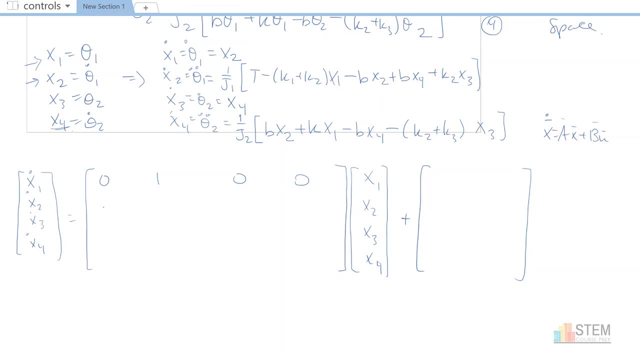 When we get there, we'll start filling it in. Now for the next one: x2 dot. for this one, remember we have this j1 here in the denominator. We're going to go through and pull off the coefficients, So we have negative k1 plus k2.. 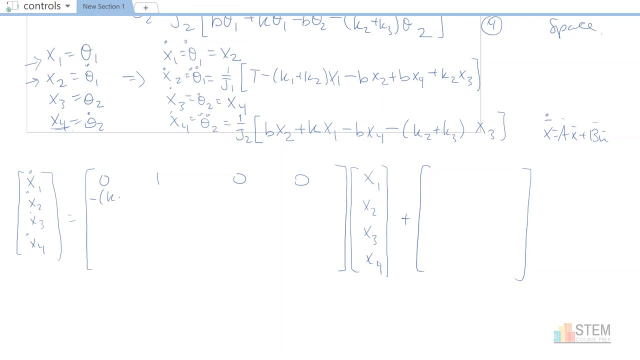 That's the coefficient of x1.. And then that's got to be divided by j1.. Now we go to the x2 term. So x2, we have negative b. We're going to divide that by j1.. That's all we have for that. 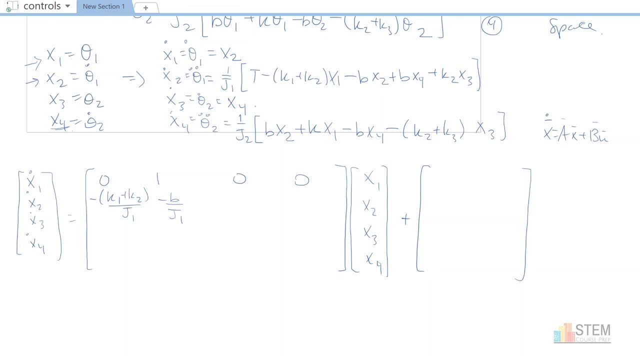 Go to the next row. And again, I'll take care of this t in just a minute. Go to the next row. We have x4.. Actually, we've got to finish this row out. We're not going to the next one yet, So let's look for x3.. I forgot. 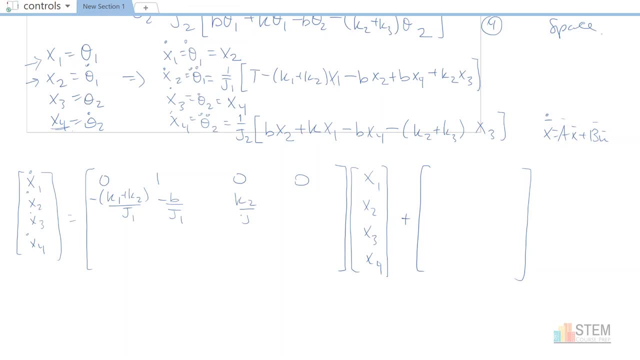 We're going to have k2 for x3.. So we're going to have k2 over j1.. And then, finally, for x4, we've got b over j1.. So this is going to be your row for the x2 dot row. 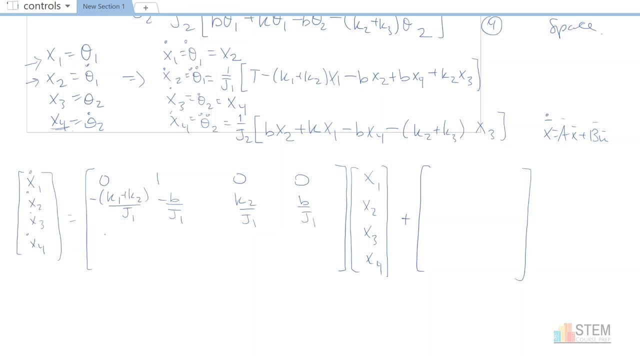 And again, I'll take care of the t in just a minute after we get done with the A matrix. Now let's go to x3 dot, where it is just x4.. So this one, we only want that one variable. So we're just going to have 0,, 0,, 0, and then 1.. 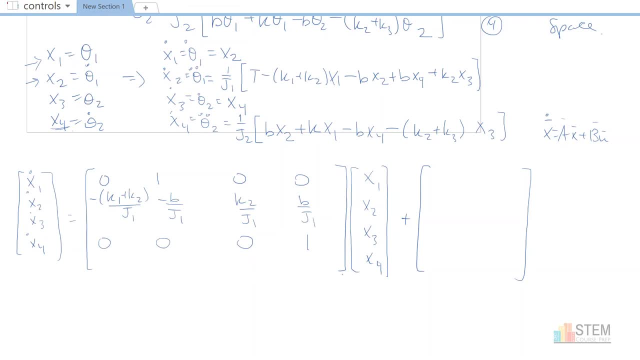 Because, again, when we multiply this row by this column vector, we're going to end up with x4, which is what we want. Next, last one here: Coefficient for x1 is going to be k. Let's see right here. So we're going to have k over j2,. 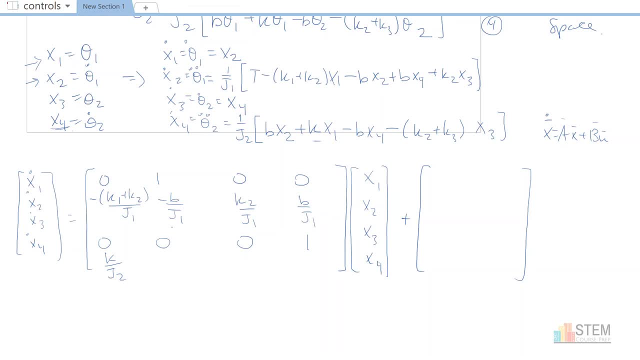 because we have this j2 at the front And then your x2 term is going to be b over j2.. x3, we have the negative k2.. k2 plus k3. With that over j2.. And then, finally, for x4, I have negative b over j2.. 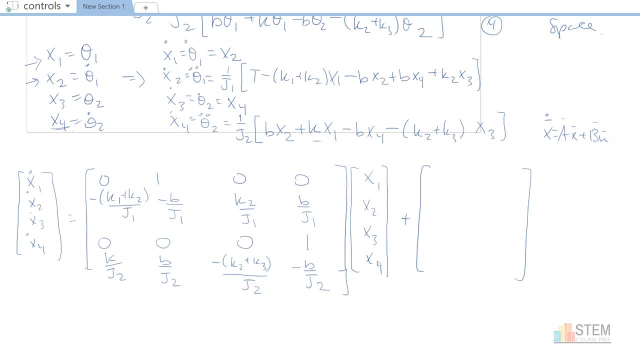 Alright, so then that is our A matrix. So we're done with that part. Now I've got to go to the b times u term right here. Now, b times u. this takes care of your inputs, So for u in this problem, u would be our input. 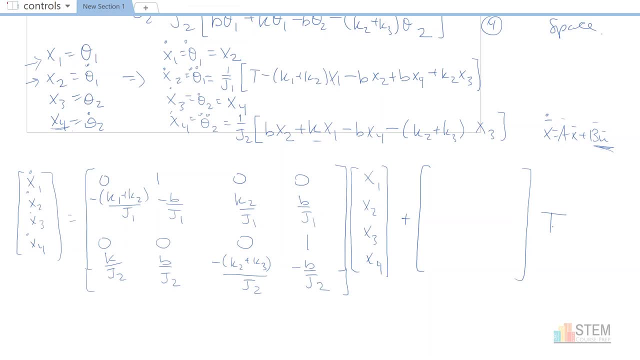 We're going to have t. t was that applied torque? We only had the one applied torque, So we just put a t here And now, basically, you're going to go through your four equations again and we're going to look for every equation that has t in it. 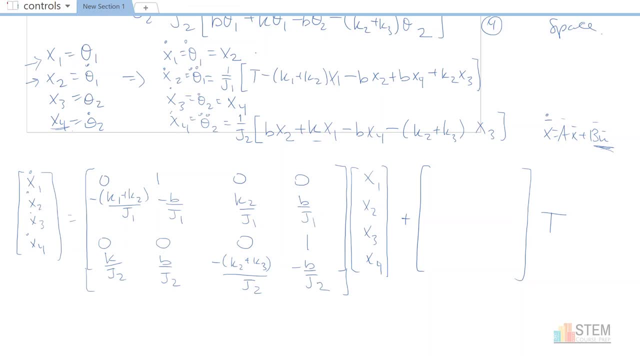 Alright, if it doesn't have a t in it, we're going to put a 0 in matrix B for that element. So for x1 dot it was just x2.. So that means this would be 0.. For the next one, I have t over j2.. 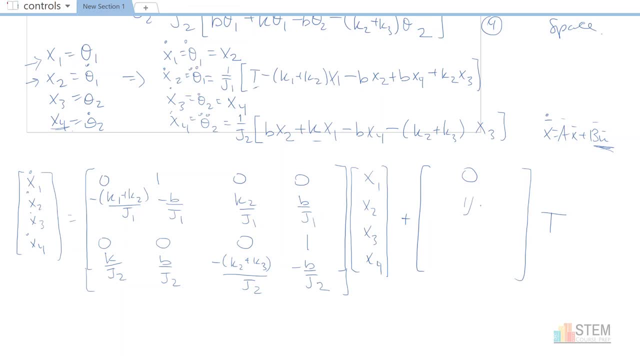 So that means this needs to be 1 over j1. Because that way when we multiply I get t over j1. So then when you do this entire equation for x2 dot, you'll do the A times x term and then you'll have plus the t over j1. 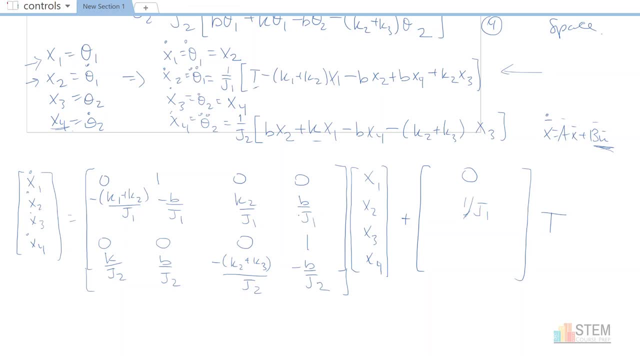 So that'll give you exactly what we had right here For x3 dot, I just had x4.. There is no applied torque here, So this would be 0.. And same thing with x4 dot: There is no applied torque. 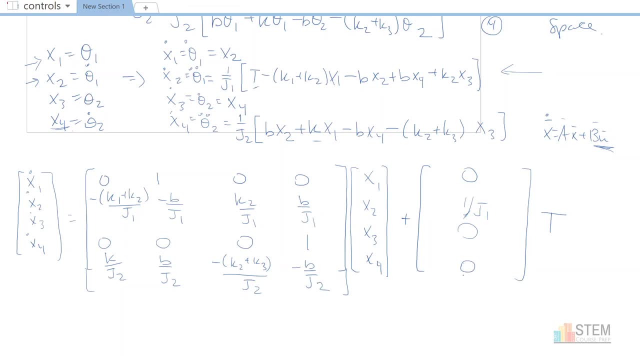 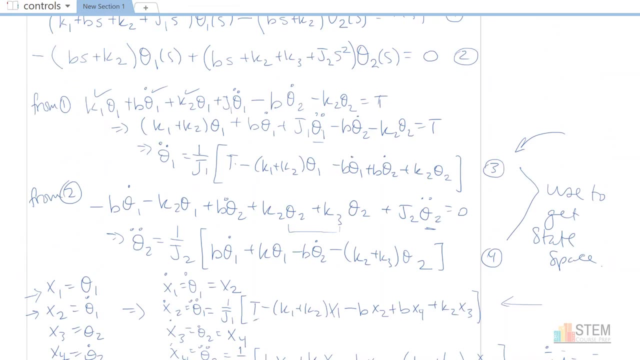 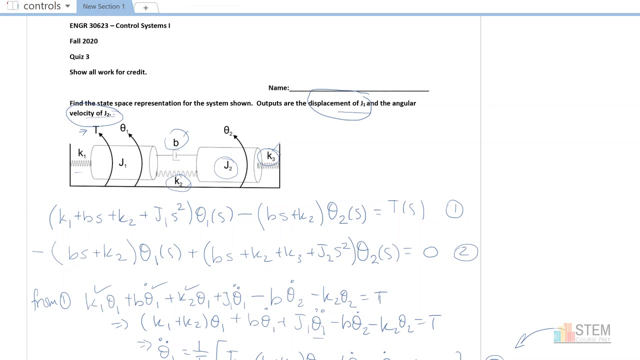 so we would just put a 0 for that one. Okay, so now we got that far, and then what we need to do now is look for our output. So our outputs: remember: we have displacement of j1, and then that angular velocity of j2.. 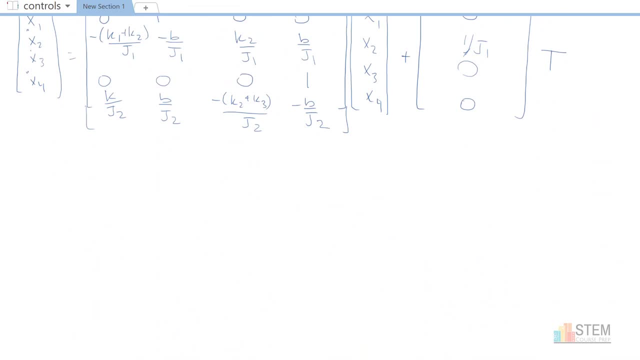 So we need to figure out what our c matrix was. So we're going to have y equals c times x. Now remember, a lot of the books have that plus du term. We don't need that for this problem, Because that's when you have coupling effects. 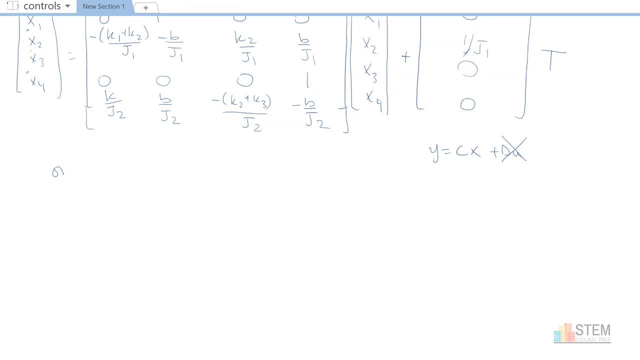 and we don't have that here. Okay, so our output is going to be displacement of j1. And then we're going to have the angular velocity of j2.. So we're going to have the angular velocity of j2.. Now what you need to do is figure out. 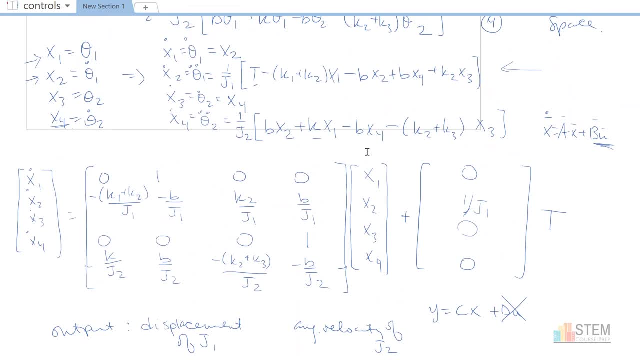 what variables represent those two things. So which variable do we have that represents the displacement of j1? Well, displacement of j1 is theta1, and our variable that represents theta1 is this x1, right here. So that means, when I multiply the c times x, 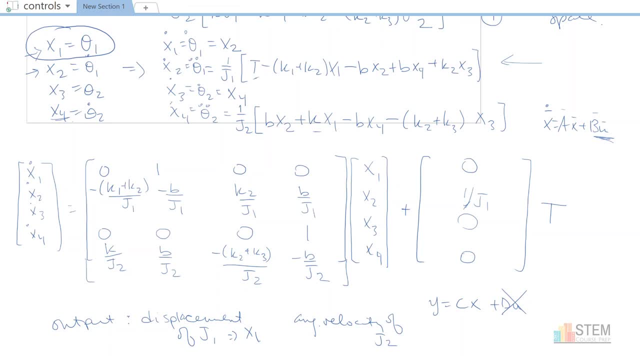 I need to get x1.. And then for the angular velocity of j2, well, the angular velocity of that one is theta2 dot. So theta2 dot is represented by x4. So we need to get x4 out. And now let's see how we do that. 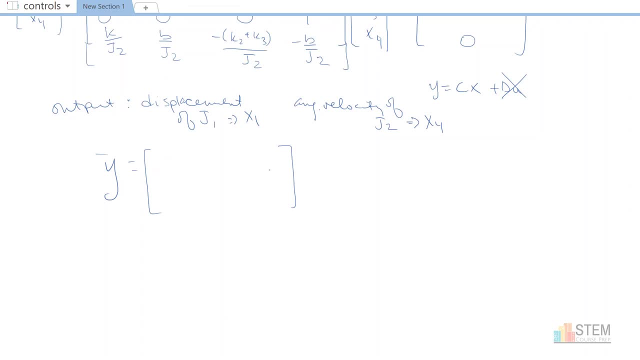 So y then is going to be vector, Vector c or matrix c times state vector again. And now I need to figure out how to get these two outputs. So I want to get x1 out. So that means I need 1, 0, 0, 0. 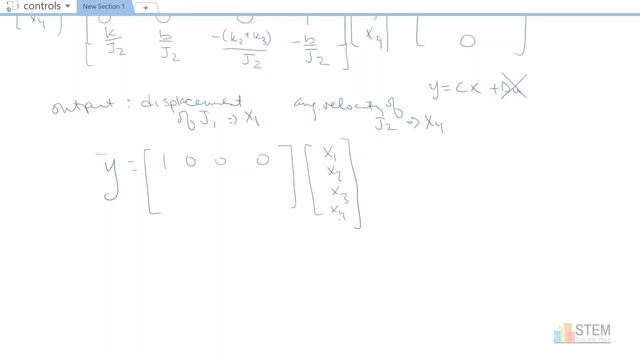 Because when I multiply this row vector by this column vector here, I would end up getting x1.. Now I also want x4. So that would mean I need 0,, 0,, 0,, 1.. and then that would give me x4.. 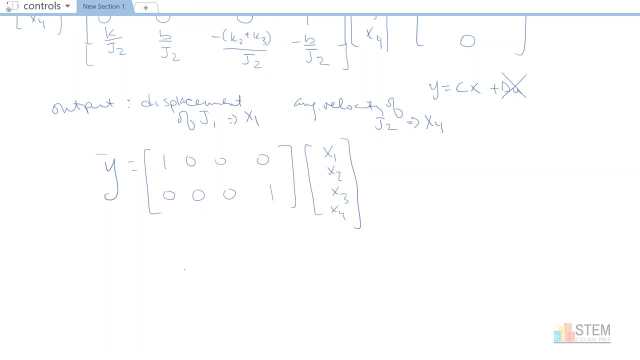 Now what you do not want to do, and I see this all the time in class. you do not want to say it's 1, 0,, 0, 1.. And the reason for that is that's giving you x1 plus x4..